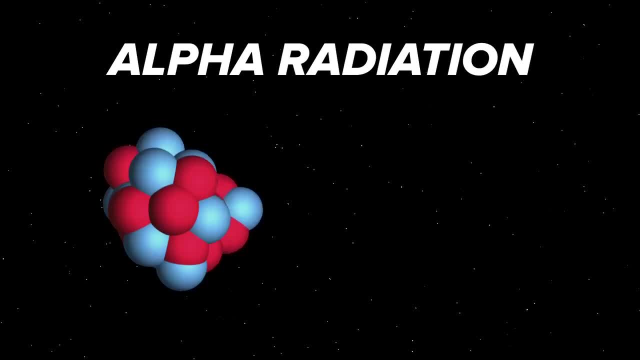 of radiation have different characteristics. Alpha radiation is when an atomic nucleus shoots out an alpha particle which consists of two protons and two neutrons. If you dust off your chemical knowledge, you'll recall the nucleus of a helium atom contains two protons and neutrons. so alpha radiation is. 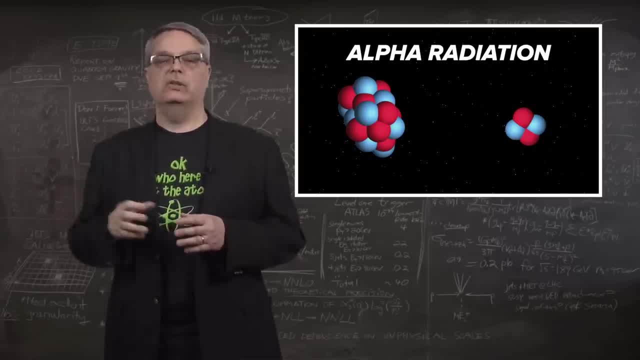 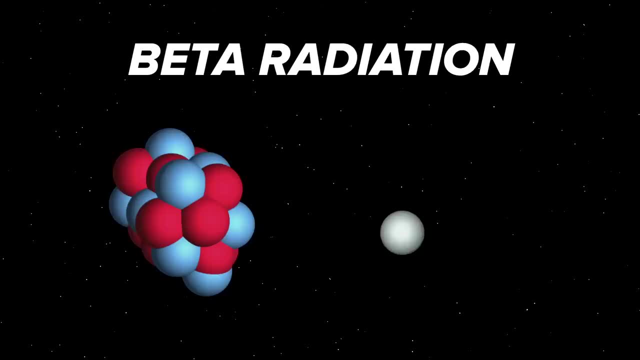 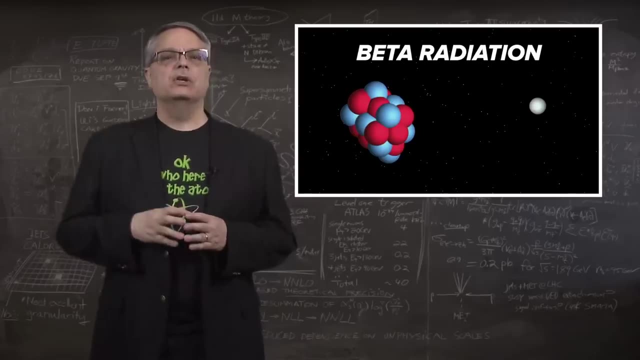 when a radioactive element shoots out a helium atom minus the electron. Beta radiation is caused when an atomic nucleus shoots out an electron. We could call it electron radiation, but the name was invented before we identified the emitted particle as an electron. It generally occurs when a neutron in an atomic nucleus turns into a proton and an electron. 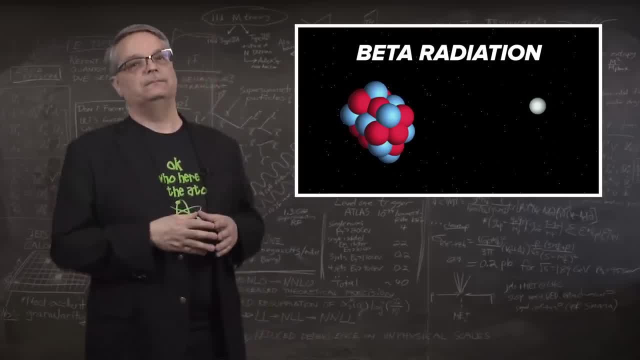 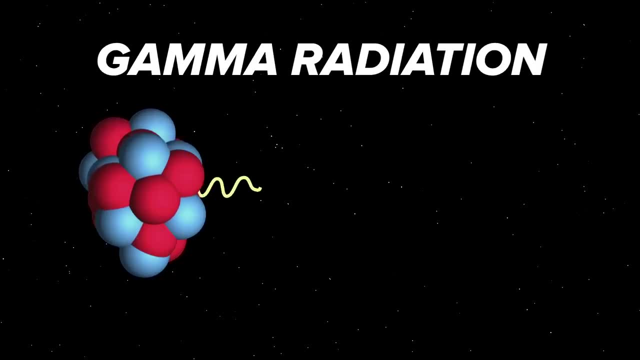 The proton is kept inside the nucleus and the electron escapes. Gamma radiation is when an extremely high energy photon escapes the nucleus. In a sense, this isn't much different than a nucleus emitting ordinary light, but the much higher energy involved means that the gamma ray can damage surrounding material. 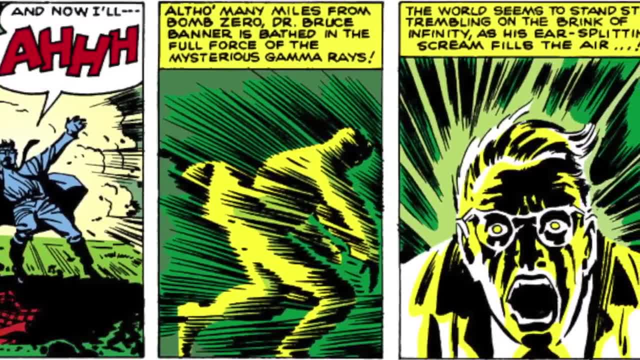 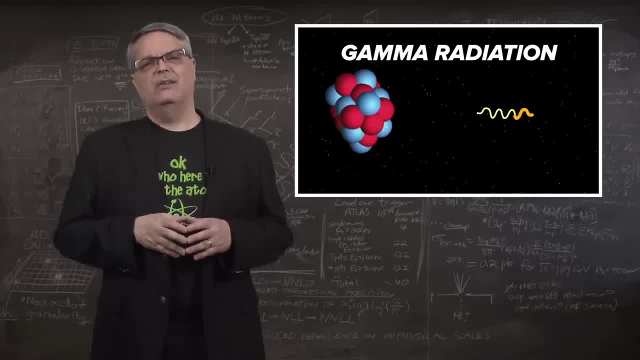 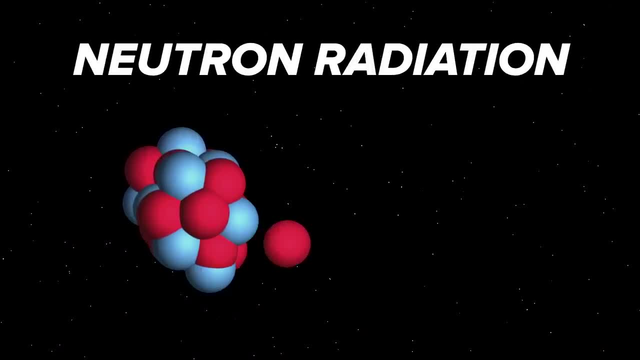 Gamma rays are often used in comic books to give superpowers to unsuspecting spectators. By the way, X-rays are similar to gamma radiation in many ways, but less energetic. They're like gamma radiation's younger and less successful sibling. And then there is neutron radiation, which is just the emission of a neutron. This is 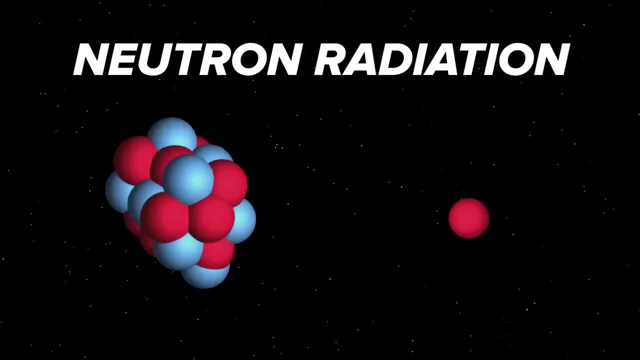 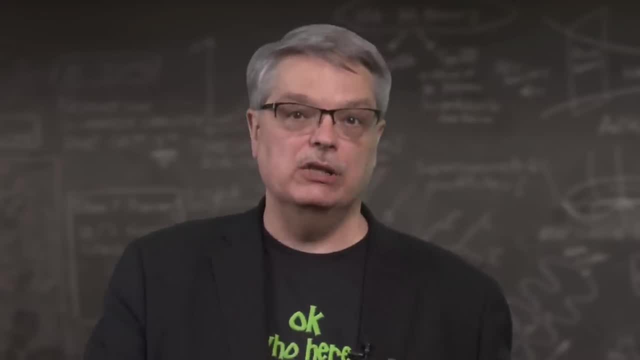 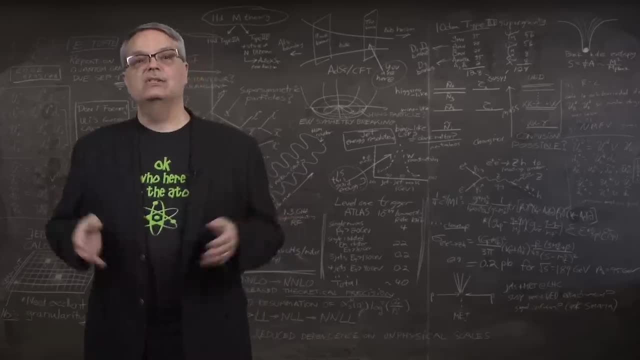 the most dangerous type of radiation, but, as we will see, that's a subjective statement. So these are the different kinds of radiation that one encounters in nuclear physics, But, as we will see, they have radically different properties. This isn't a radiation safety video, but it's important to know, at least broadly. 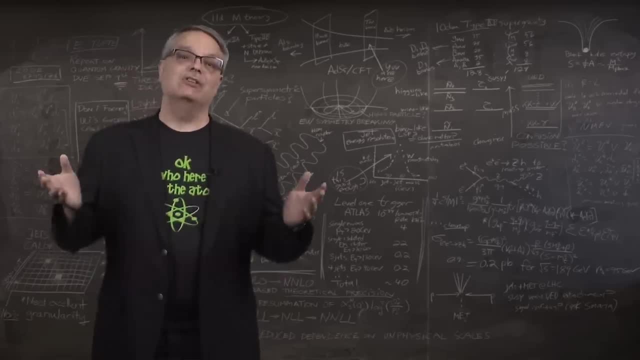 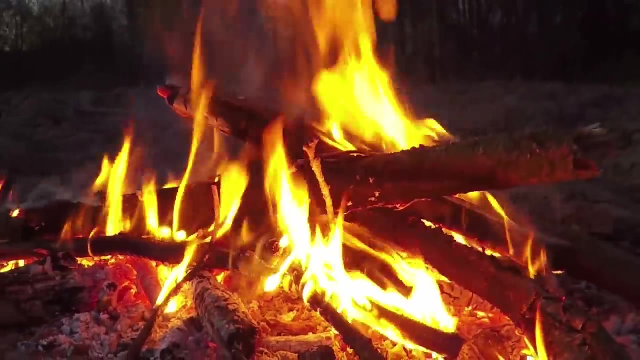 what you need to do to be safe around radiation. Perhaps obviously the easiest thing to do is just get very far away from it, Just like a fire seems cooler the further you get from it. distance is the easiest way to reduce your exposure to radiation. 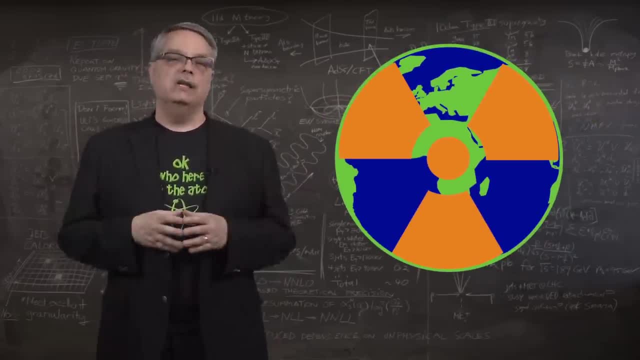 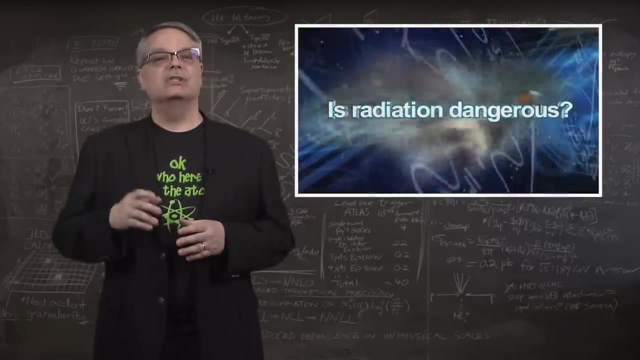 However, that's not always possible. We live in a radioactive world. Bananas are radioactive, as are Brazil nuts. Heck, you are radioactive. I made another video discussing levels of radioactivity and if you watch that, you'll understand that low levels of radioactivity. 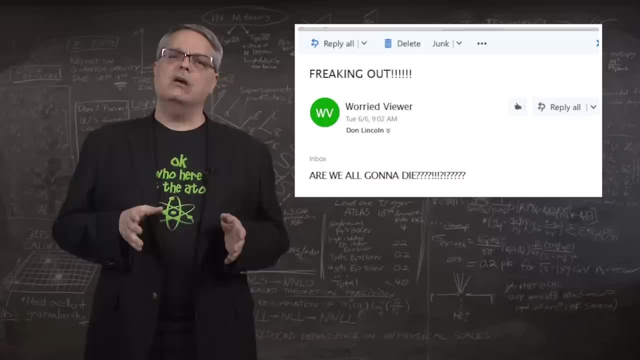 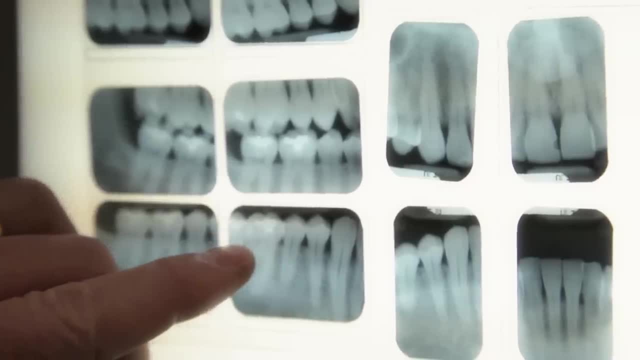 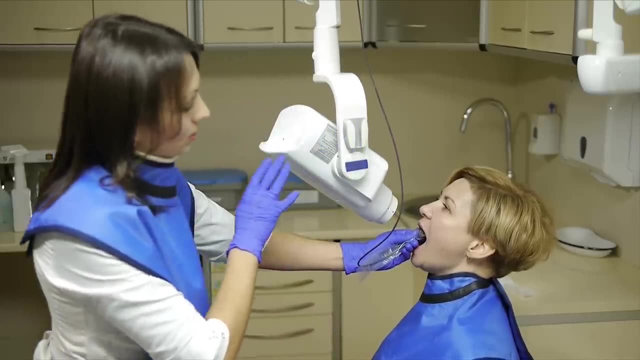 There are other types of radiation, things like dental x-rays, for example. Now, don't worry about dental x-rays. They give you a very low dose and they are definitely worth having, But if you're, for example, a dental hygienist, you might encounter lots of x-rays. 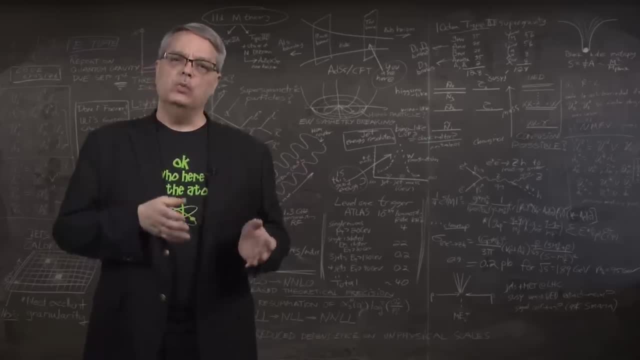 and want to protect yourself, So it's important to know about the ways in which you can shield yourself from various kinds of radiation. Alpha radiation consists of heavy and slowly moving particles with a lot of electrical charge. These properties combine to make them easy to stop. 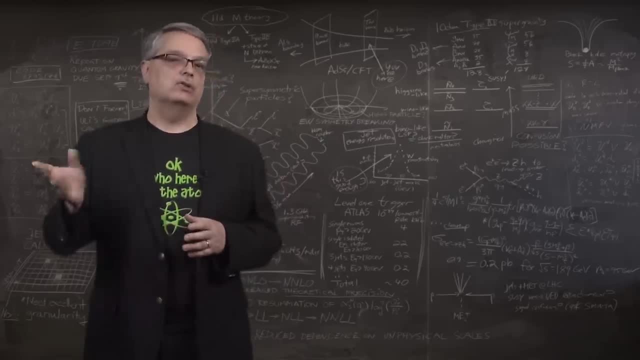 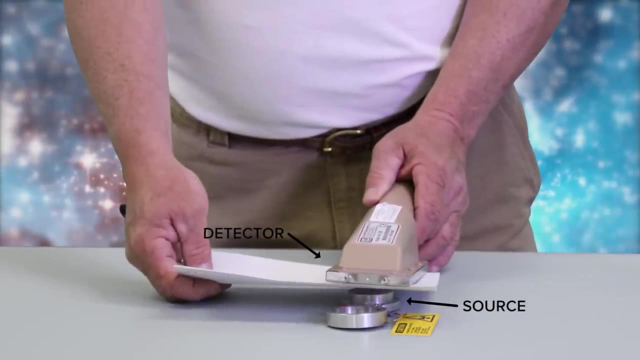 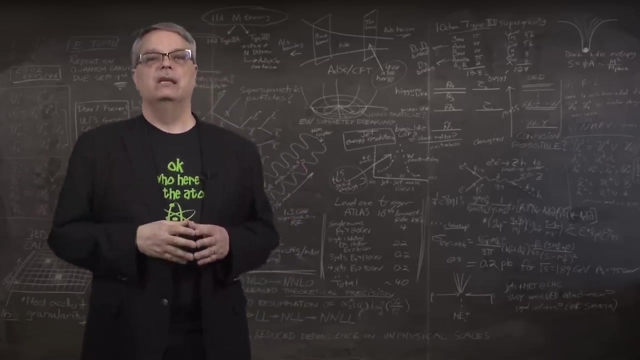 You can stop alpha particles using a single sheet of paper. Here I'll show you. Here is a sample that emits alpha particles in a Geiger counter. The paper stops the radiation. Beta radiation consists of light and fast moving particles with electric charge. 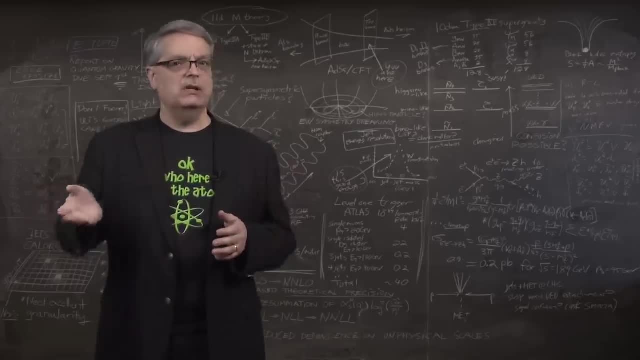 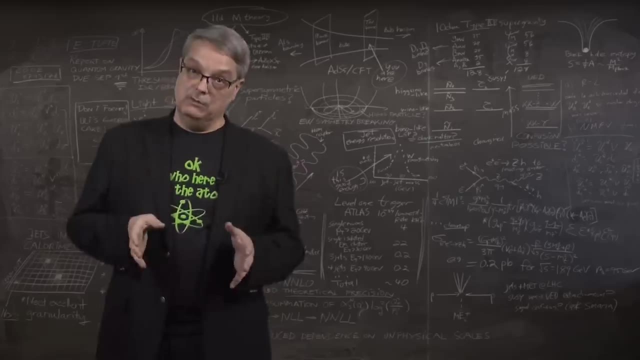 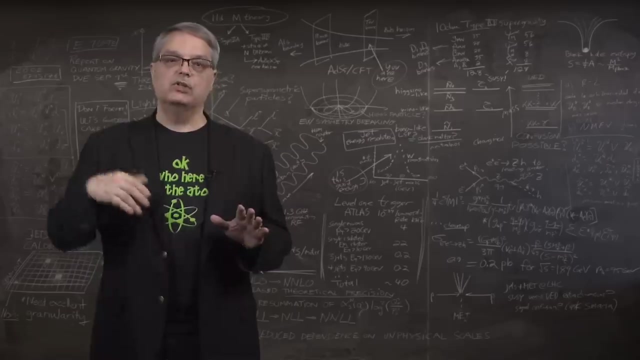 This means that they can be stopped by reasonably thin plates of material. For instance, we see here that they can be stopped by a thin metal plate. Gamma radiation consists of fast moving particles with no electric charge. This means they emit no electric fields to interact with matter. 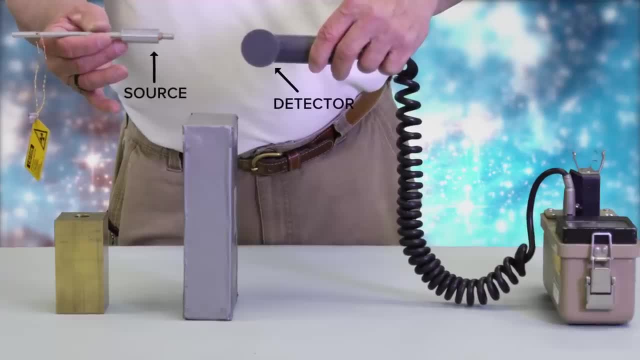 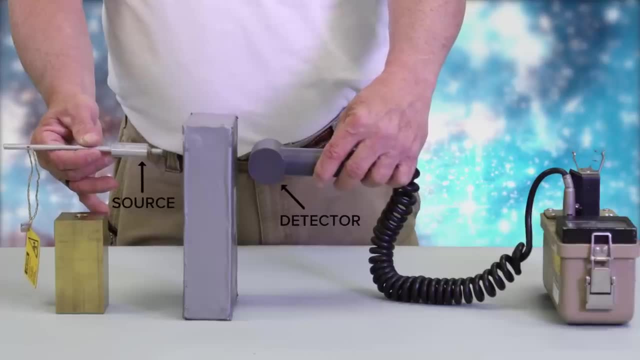 They are therefore much harder to stop. To stop gamma rays, you need a heftier chunk of dense material like lead. This is also true for x-rays, which is why they put a lead apron on you when you're getting dental x-rays. Neutron radiation consists of pretty heavy particles with no electric charge. Since they don't interact with atomic electrons, they can travel long distances, say hundreds or even thousands of meters in air. The way to slow them down is not so intuitive. You have to use something with a lot of hydrogen in it, like water or plastic. 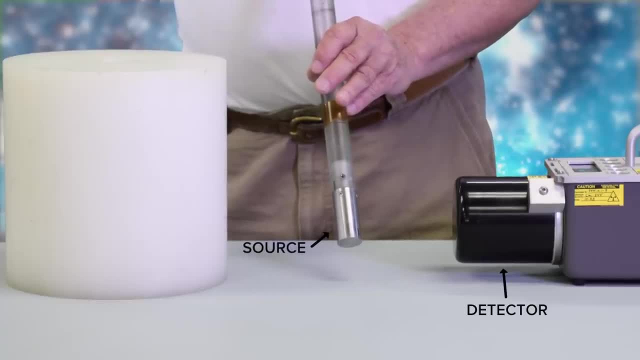 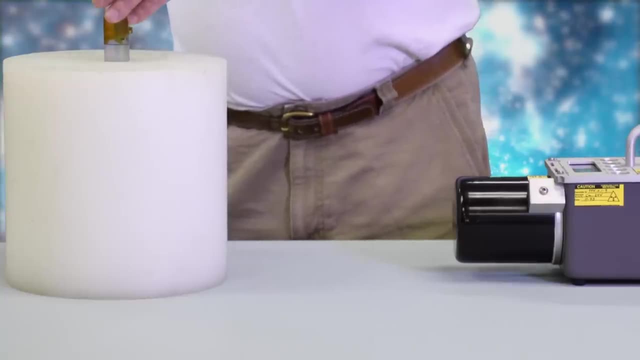 The neutrons hit the protons in the hydrogen nuclei and knock them out. This stops the neutrons and then the charged protons are stopped quickly, much like alpha particles are. By the way, given the clicking noises you heard, you might be wondering if the technician 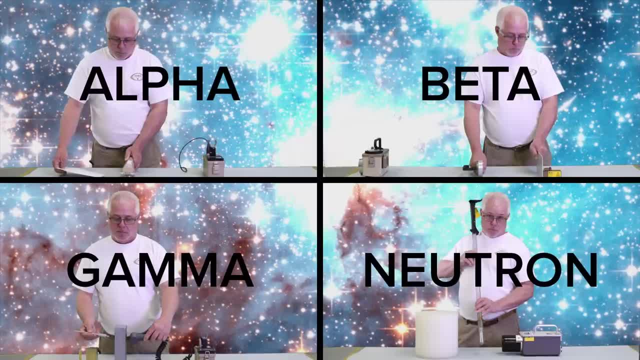 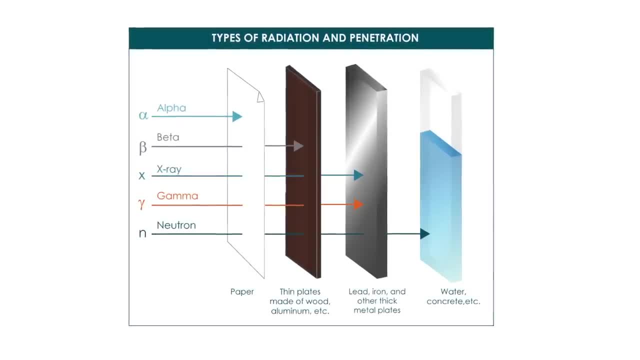 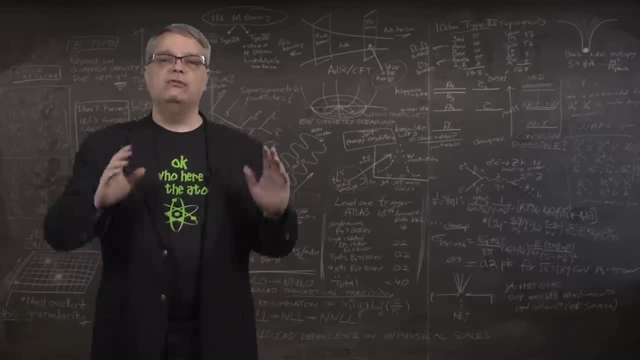 doing the demos here was in any danger. The answer is no. The radioactive sources we used were real, but they were weak. This diagram shows you roughly how to shield the various kinds of radiation. It summarizes what I just said, So I've told you about how to protect yourself from radiation, distance and shielding. 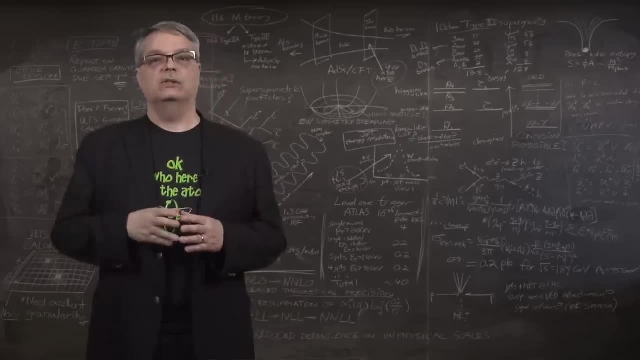 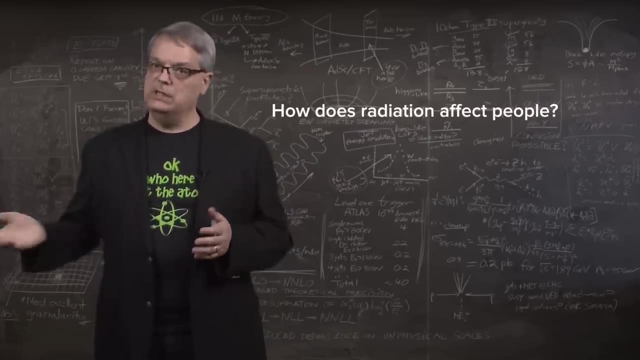 And for shielding. I've told you what works for what kinds of radiation. I hope you enjoyed this video. But what if you can't move away or get shielding? What impact do these types of radiation have on human tissues? This is kind of interesting. 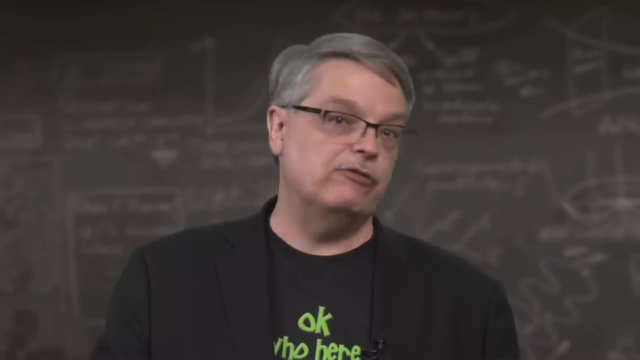 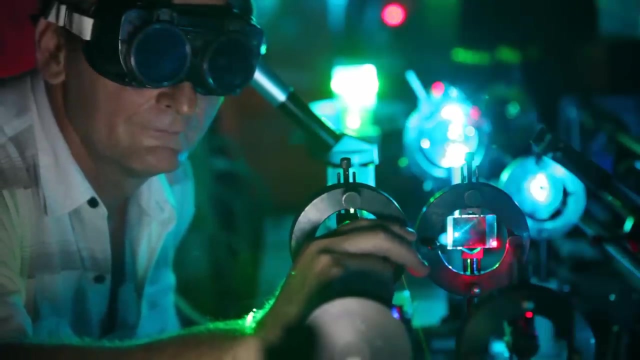 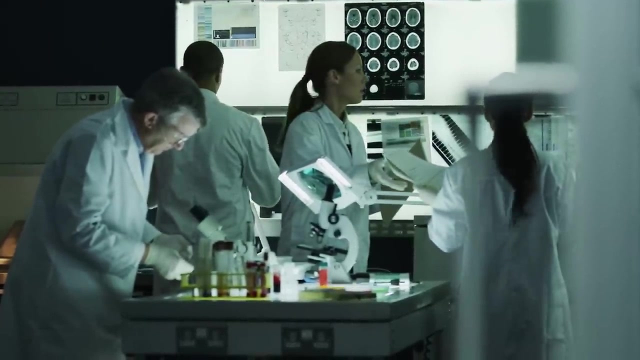 It turns out that the different types of radiation have distinctly different consequences in terms of biological damage. In order to figure this out, scientists took different kinds of radiation and aimed them at various kinds of tissue and saw how much biological damage occurred. They then came up with a number that would be used to measure how much biological damage. 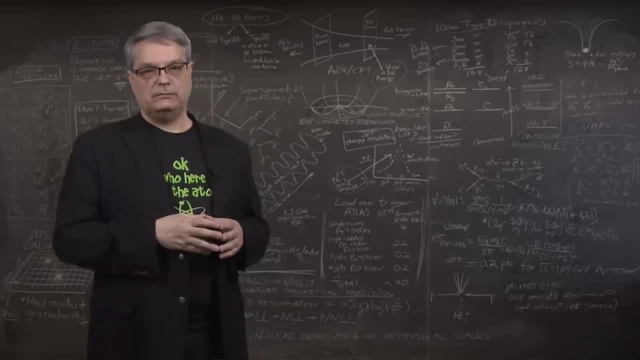 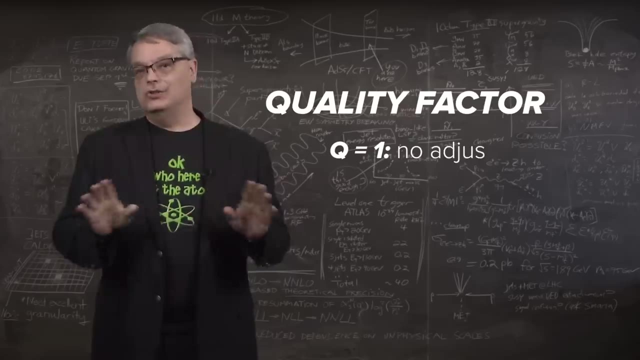 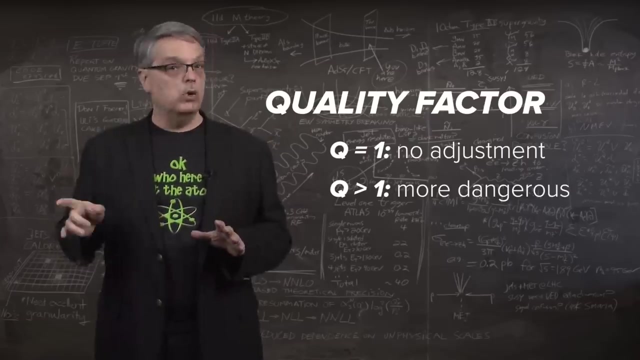 occurred. This number is called a quality factor, or just Q. If Q is 1, that means there is no adjustment. If Q is greater than 1, that means that this particular kind of radiation is biologically more dangerous than other types of radiation. 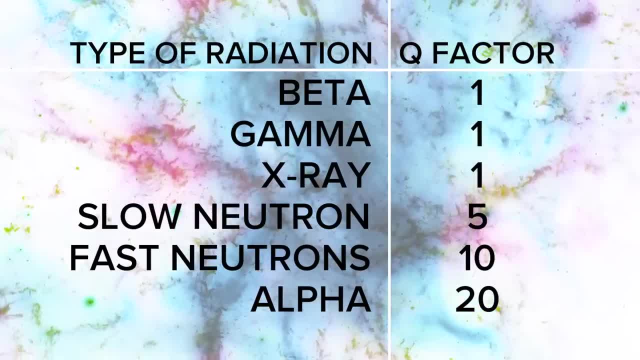 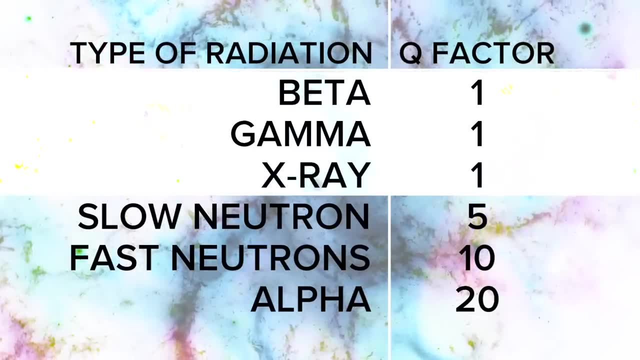 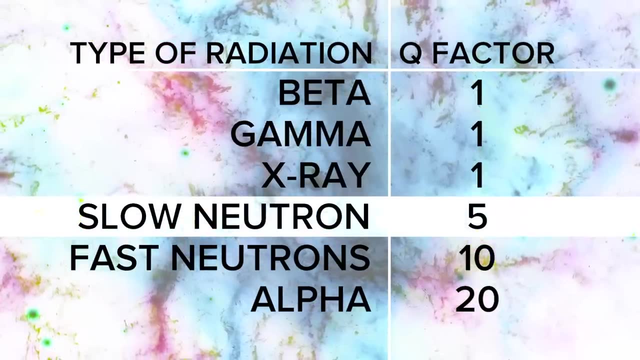 So we see here a chart that shows the Q factor for different kinds of radiation. We see that gamma and beta radiation in X-rays have a Q factor of 1. Which means that they don't have an enhanced damage capability. But slow neutrons have a Q of 5, which means that for the same amount of absorbed radiation, 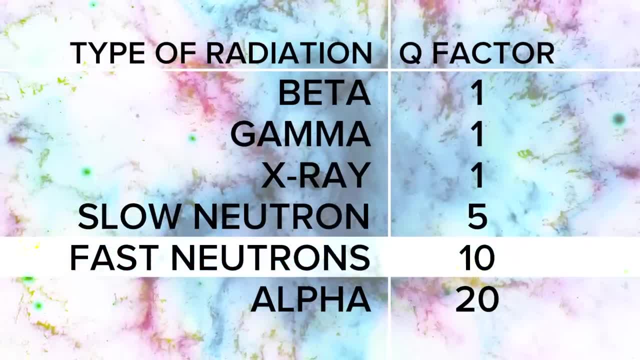 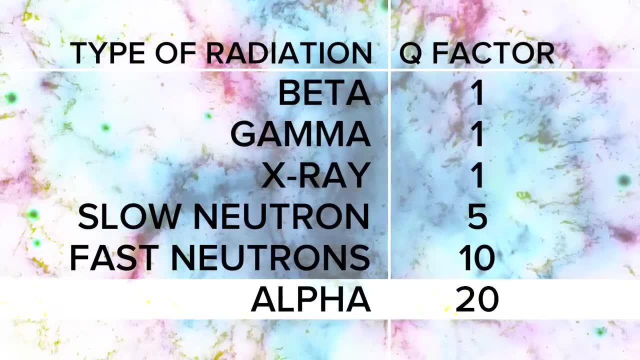 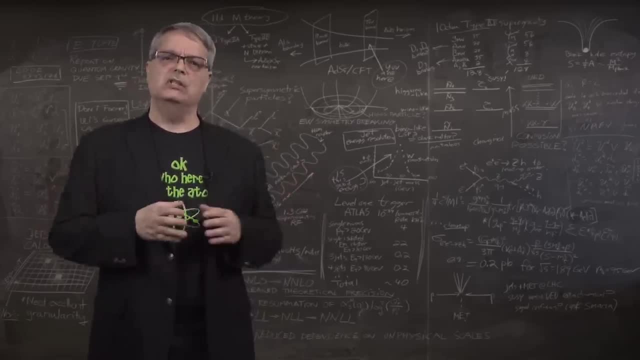 more biological damage occurs Fast. neutrons have a Q of 10, and alpha particles have a Q of 20, which means that they do more biological damage than other kinds of radiation. That last one is kind of weird. I mean, alpha particles are easy to stop but do more damage in living tissues. 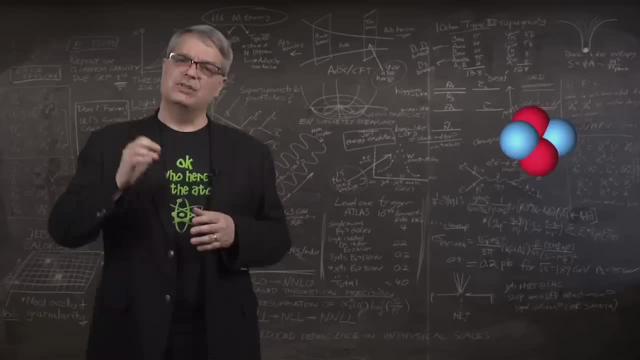 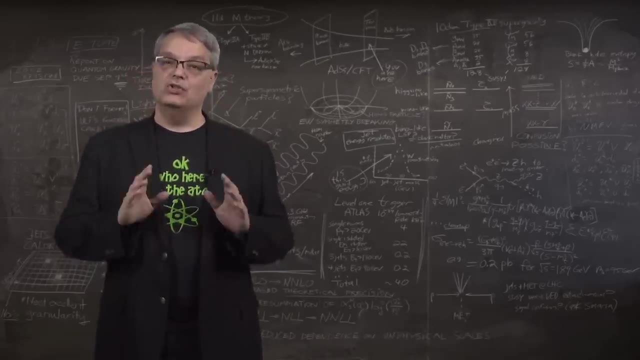 But if you think about it, this makes sense. When an alpha particle stops, it stops hard and it deposits all of its energy in one place. This means when it hits a cell, the local damage is extensive. This is especially true if you're unlucky enough to inhale alpha-emitting radioactive. 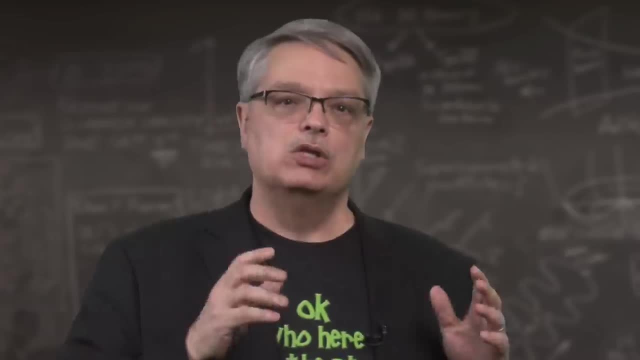 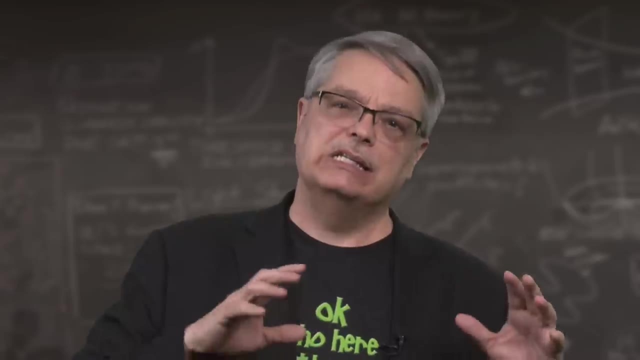 dust. That's extremely dangerous. So I hope that this video kind of gives you an idea of the diversity of possible kinds of radiation. I mean, there isn't a single kind, and that means that if you want to understand radiation and how to react in a certain situation, you need to know what radiation is.